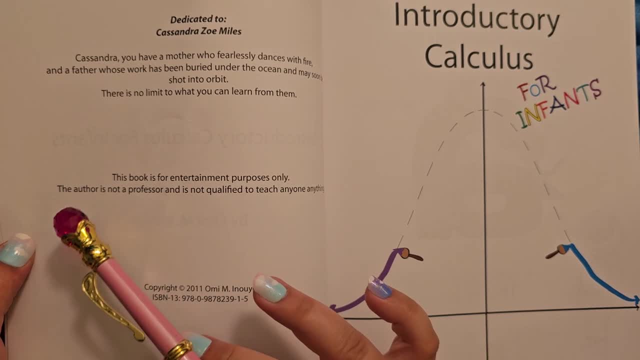 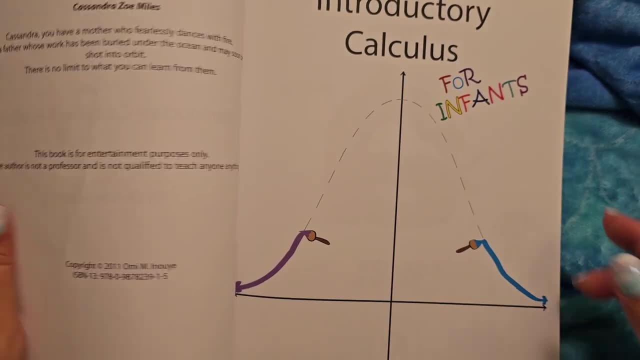 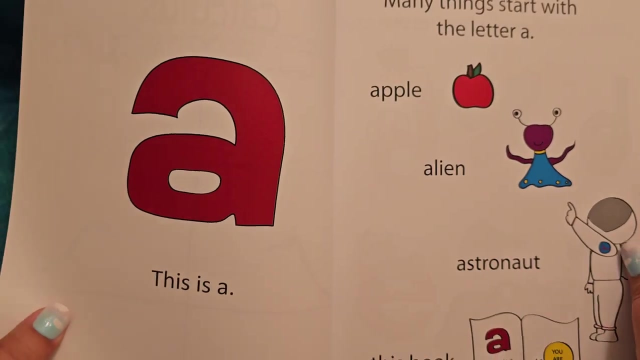 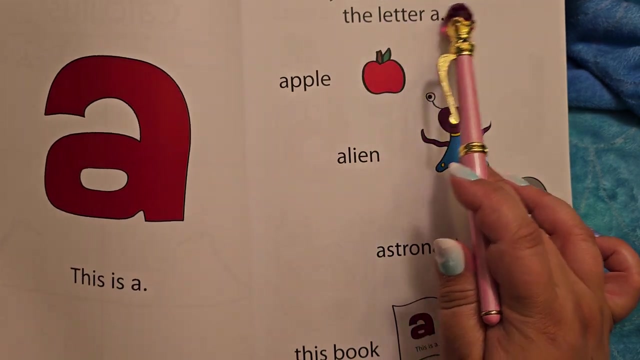 This book is for entertainment purposes only. The author is not a professor and is not qualified to teach anyone anything. I don't know about that, but all right, Introductory Calculus for Infants. How colorful A This is. A Many things start with, oops, the letter A Apple. It's a red apple. 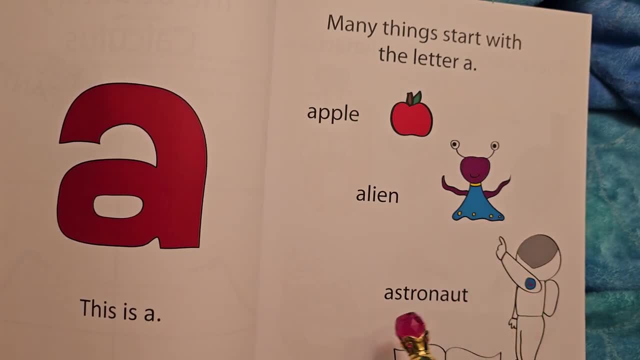 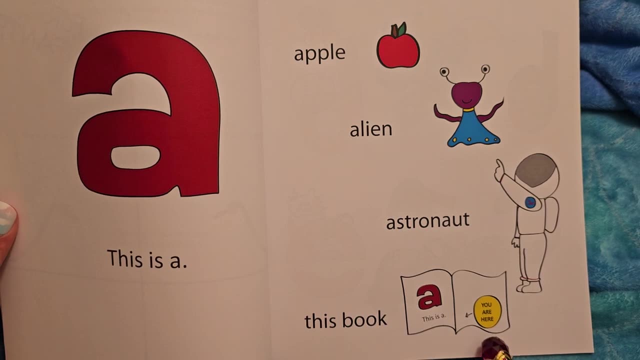 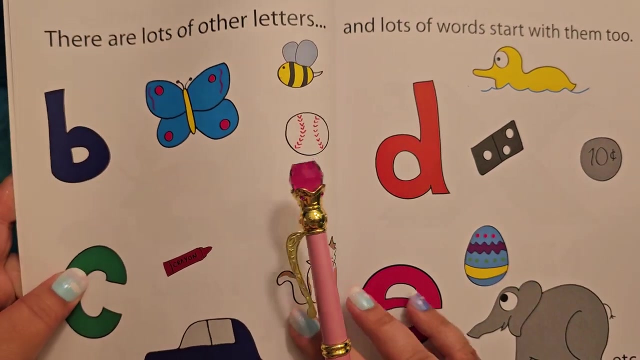 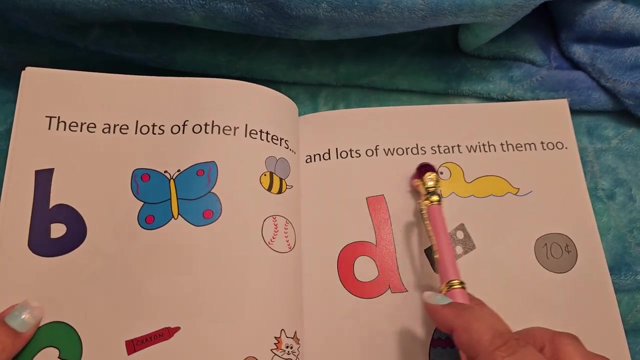 Alien- Oh, it's a purple and blue alien with a blue dress Astronaut. Oh, he's pointing to the alien because he's going to the space. This book, A. This is A. You are here, Fairy. There are lots of other letters and lots of words. Start with them. 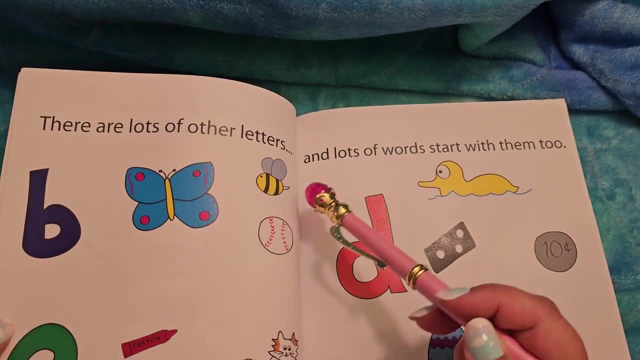 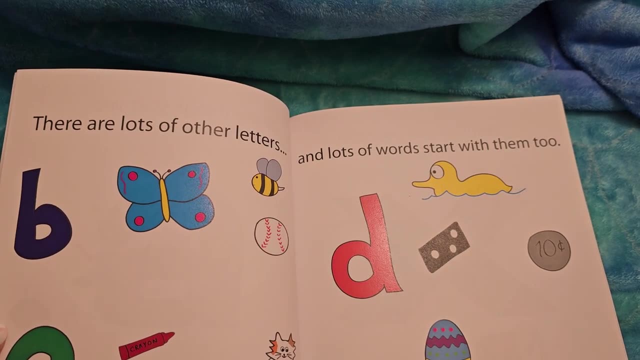 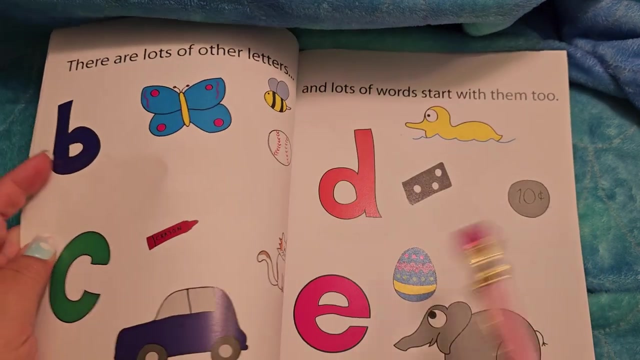 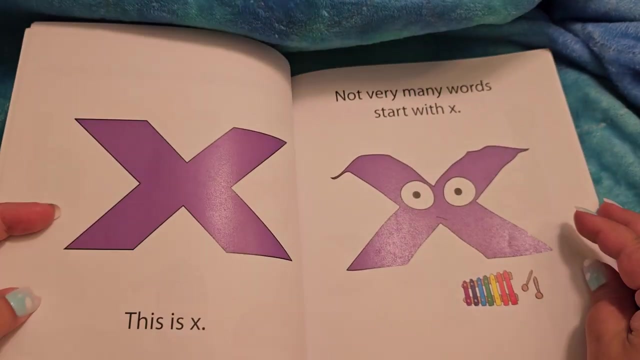 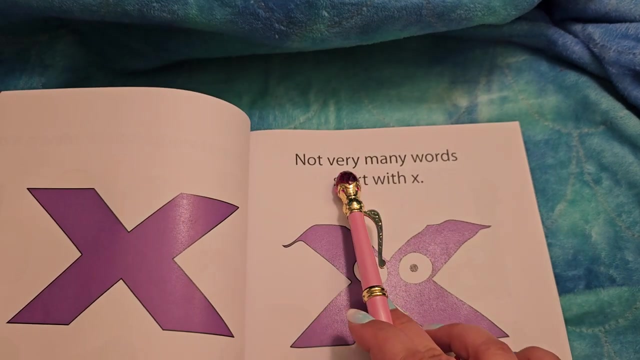 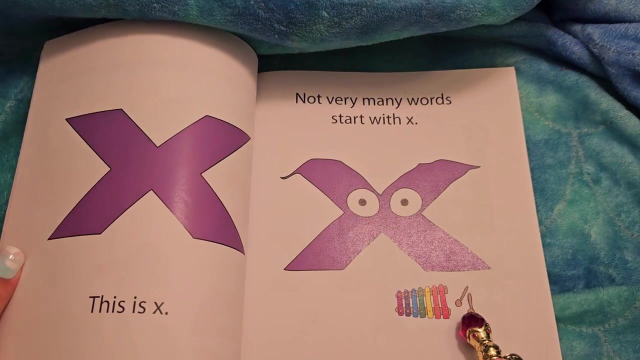 too. So B for butterfly and B and ball Bzzbzz, C for crayon and cat and car, D for duck and domino and dime E-woops- for egg and elephant, elephant, etc. X, This is X. Not very many words start with X. It's a xylophone, I don't. 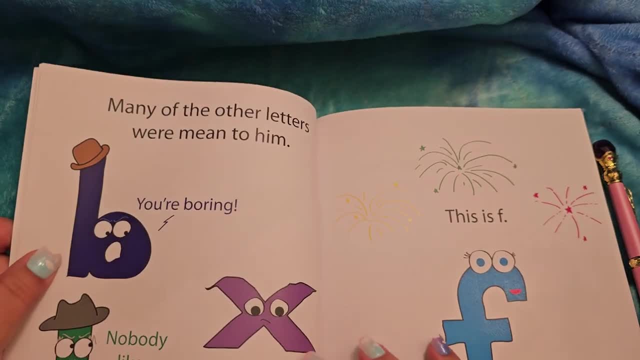 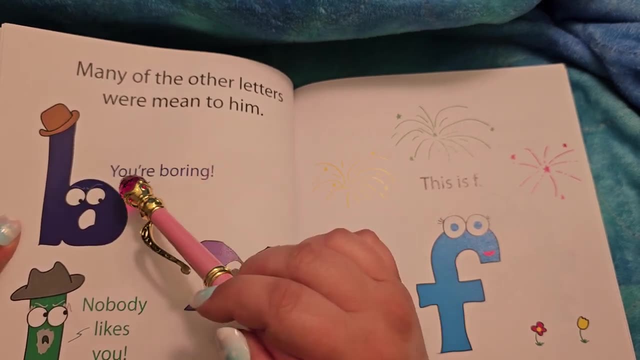 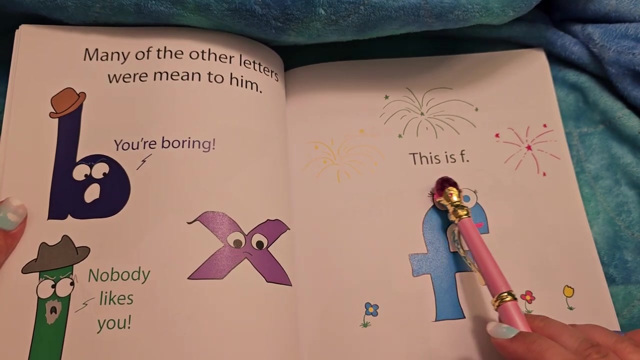 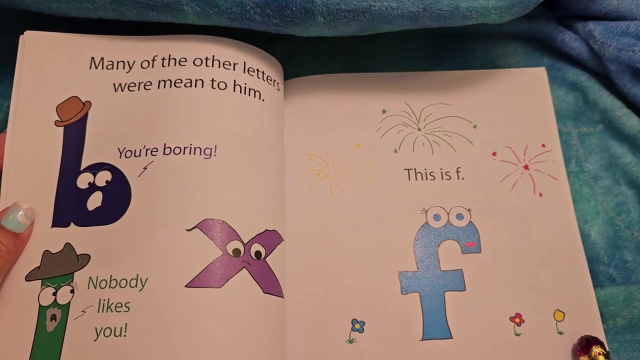 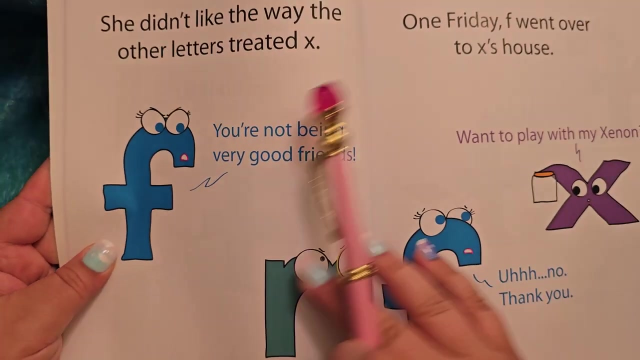 think X likes that. he's less popular, potentially. Many of the other letters were mean to him. Aww, you're boring. That's so mean. Nobody likes you. Oh, my goodness, poor X. This is F. She is fabulous and fun, Ooh, and there's flowers and fireworks. She didn't like the. 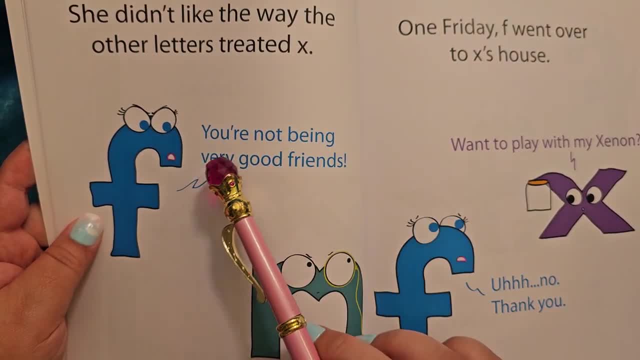 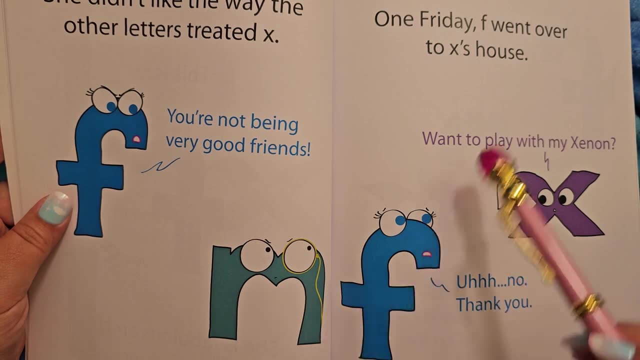 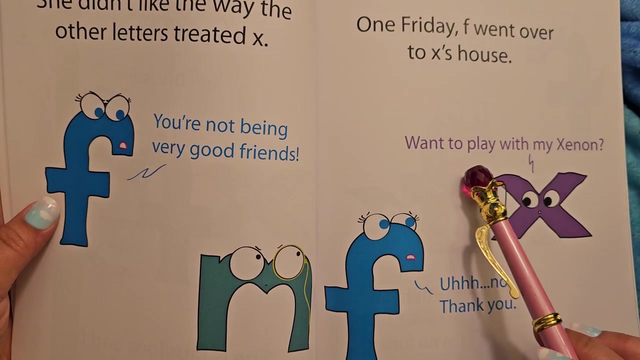 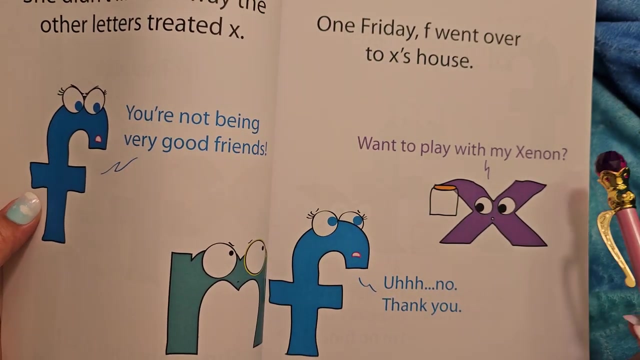 way the other letters treated X. We're not being very good friends. That's what she's saying to M here. One Friday F went over to X's house. Want to play with my Xenon. Ooh, that is a guess. Ah, no, thank. 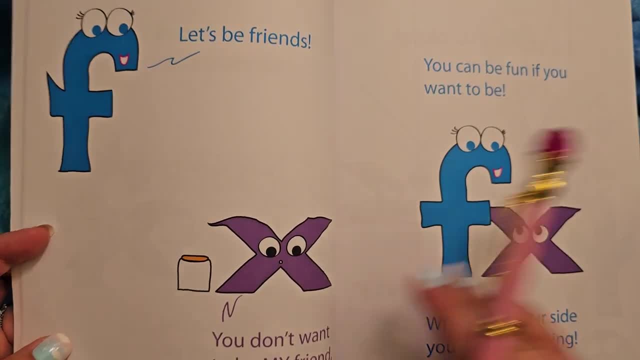 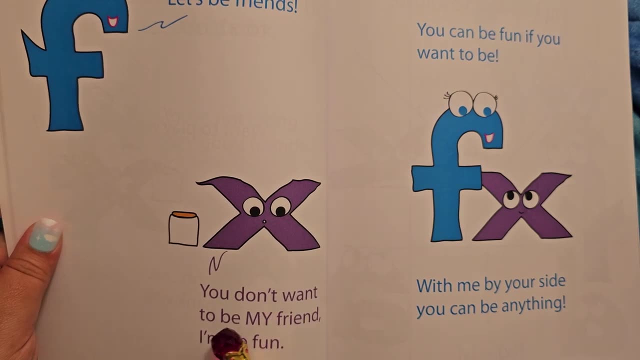 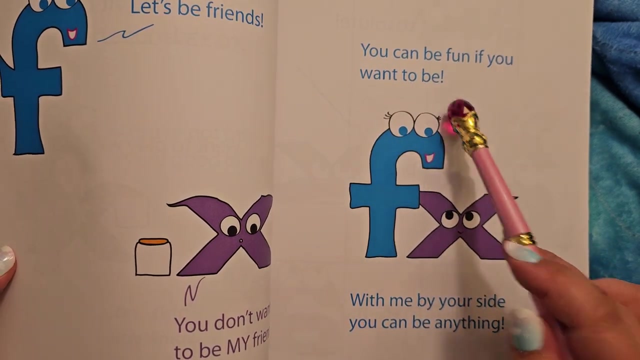 you See, that's what you say. if you don't want to do something, You're polite. Let's be friends. you don't want to be my friend? I'm no fun. you can be fun if you want to be with me by your side. you. 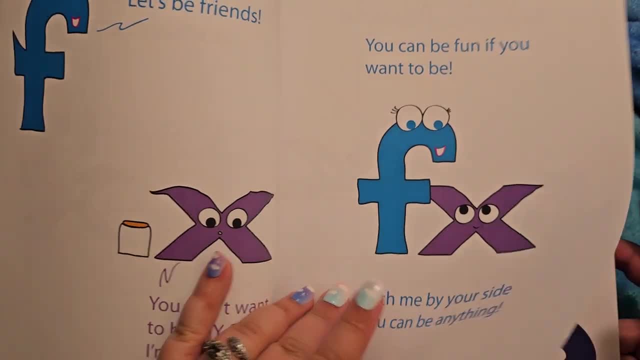 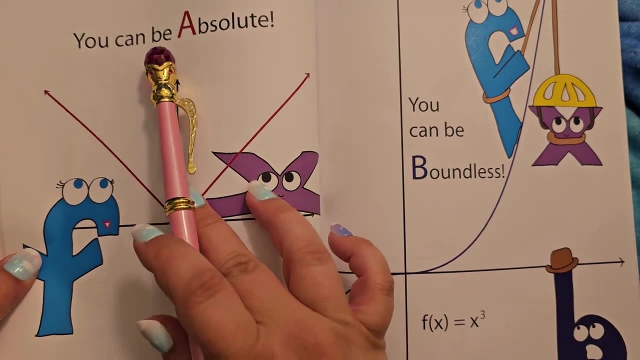 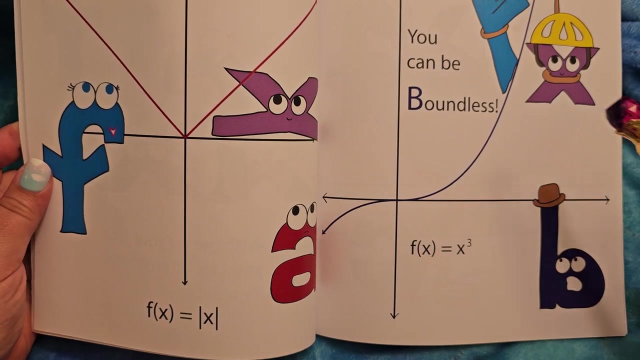 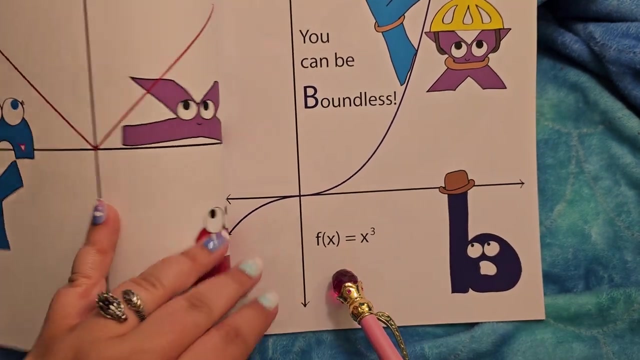 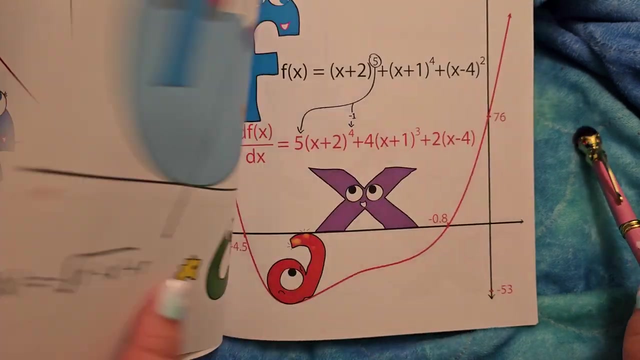 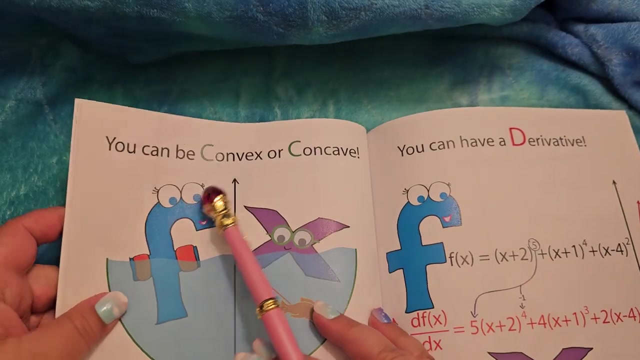 can be anything. you can be absolute, so F to X is an absolute X. you can be boundless, so FX could equal X to the third. that's what that means. looks like she's climbing up with climbing gear. that's fun. you can be convex or concave. 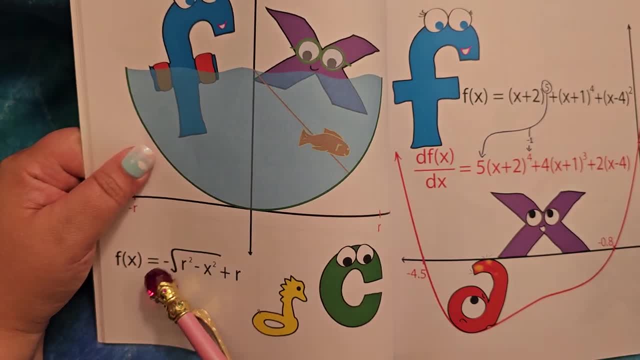 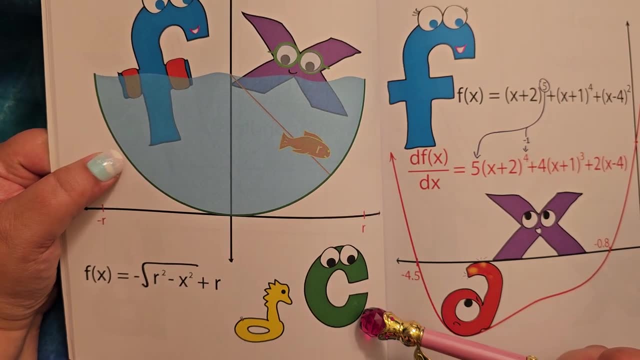 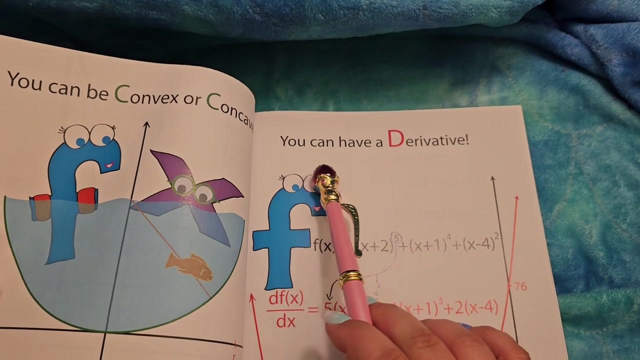 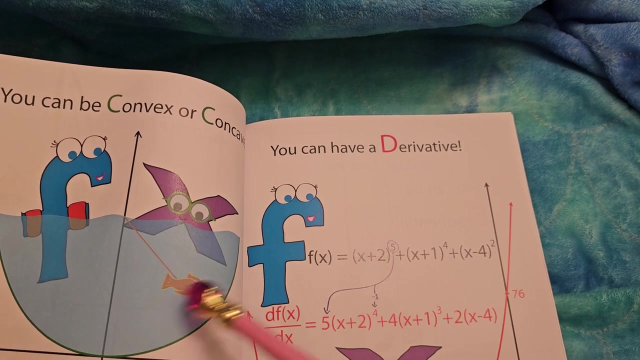 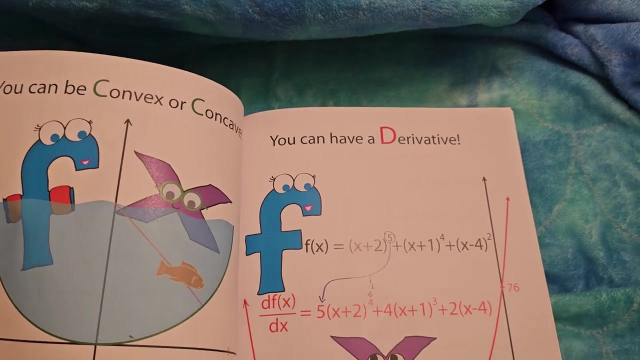 oh, look at this one FX. so the square root of R squared minus X squared plus R, so your C over here, looking a little bit down, you can have a derivative. that's a math term: convex, and concave has to do with the direction. so convex means it curves away, concave means it curves inward. oh, look at all of this fun. 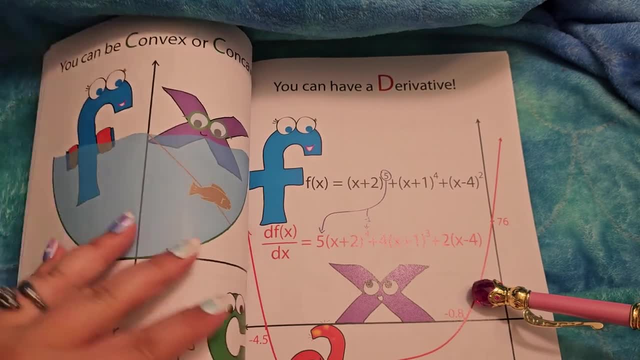 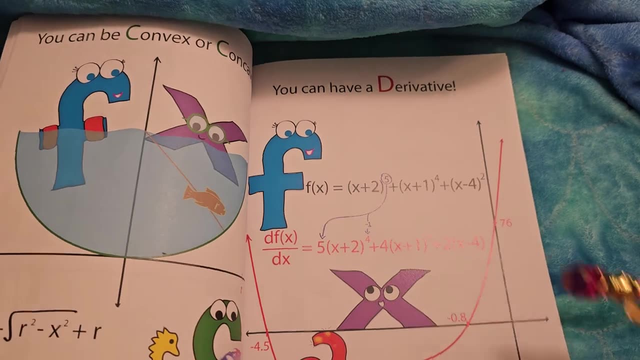 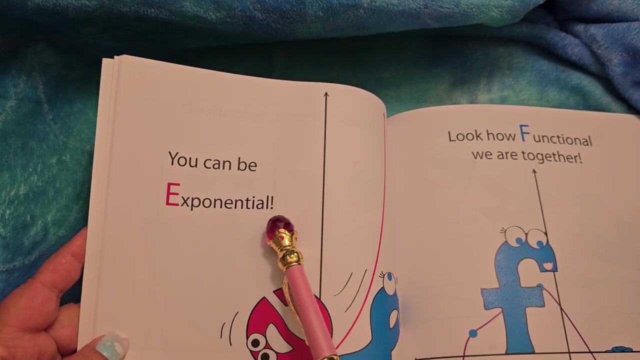 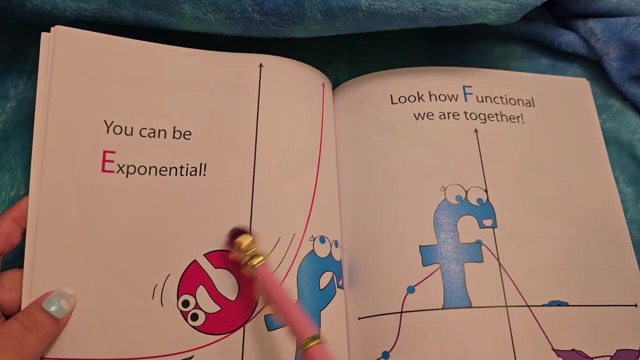 this is a. there's a lot of math. I'm not gonna read this one aloud, but that's a derivative. as a way to to break things down, that's a little chart there. you can be exponential. oh so E to the X. before E is falling down. look how. 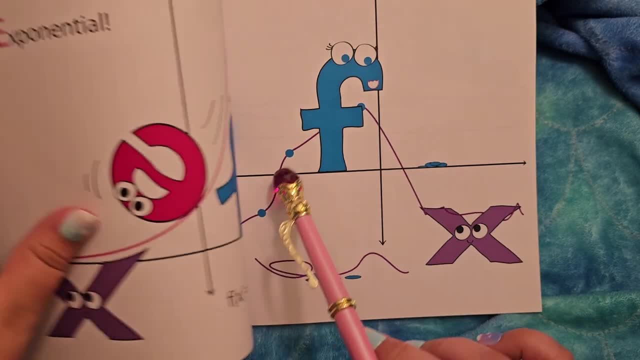 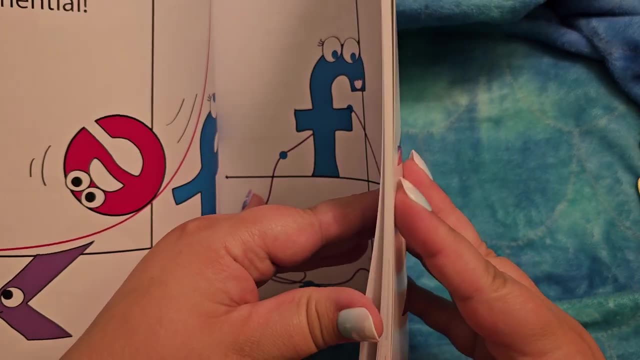 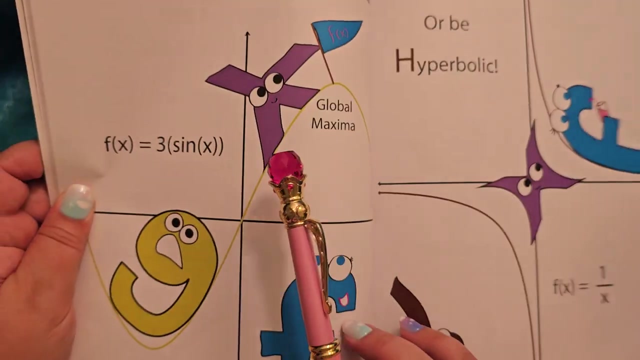 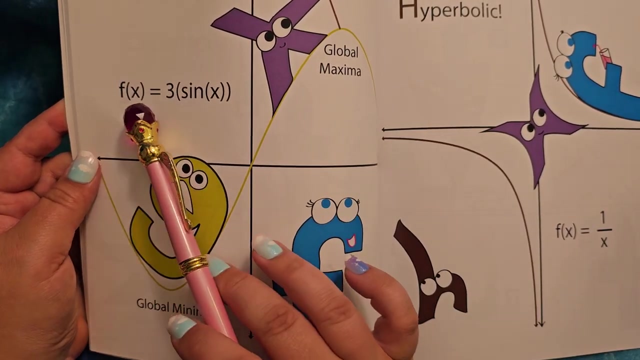 functional. we are together. oh my goodness, I I don't know how functional they are, but sure, cool, it's a function. you can have global extrema- and I'm probably saying that wrong- global maxima, global minima. so after the X is three, is sine of the X or be hyperbolic. 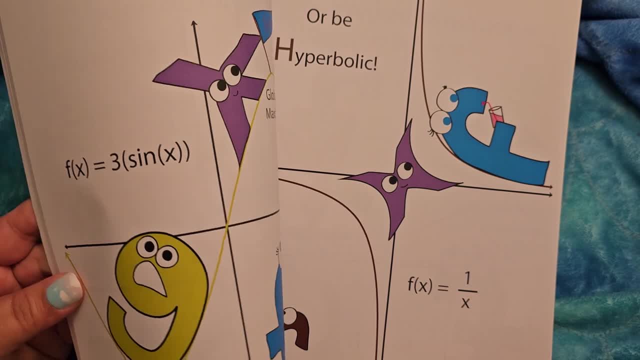 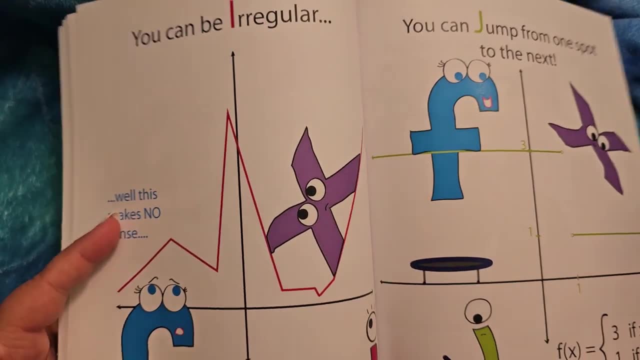 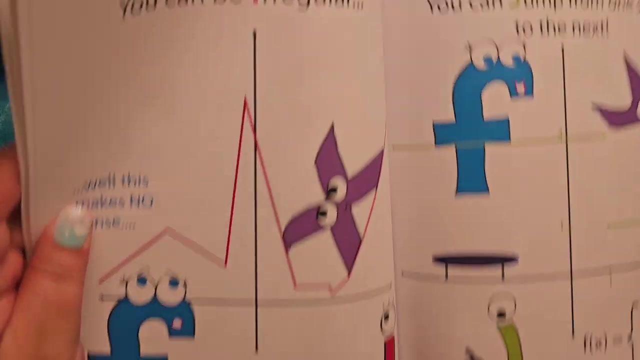 little H is looking a little nervous there. I almost feel most the letters are looking a little unhappy. look at the G. that's the X of 1 over X. you can be regular. well, this makes no sense. who knows what's going on here, but I seems. 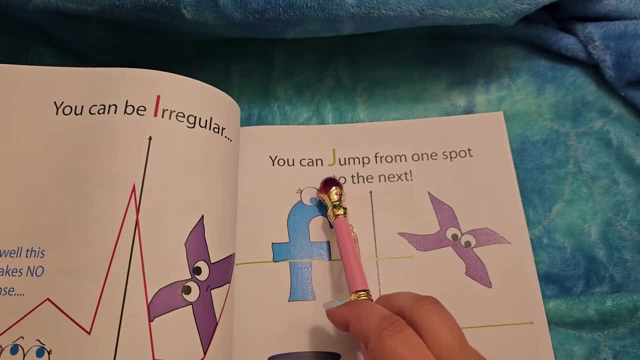 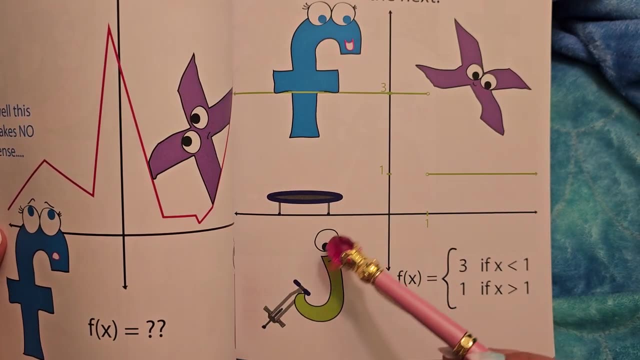 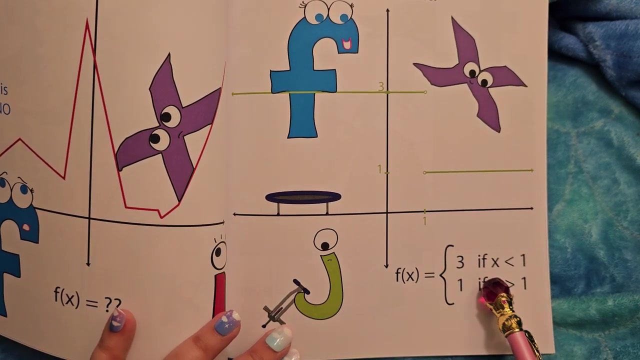 interested. you can jump from one spot to the next. little trampoline, boom, boom, and the J is got a little pogo stick, so he's jumping. so look. so F of the X, 3 is if X just less than 1 and 1 if X is greater than 1. 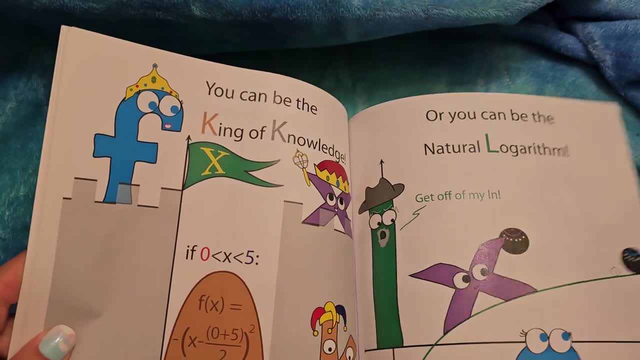 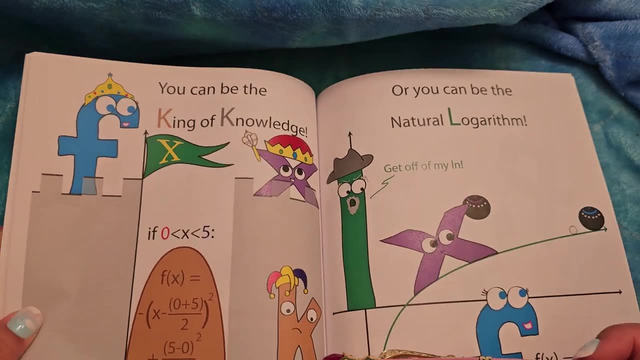 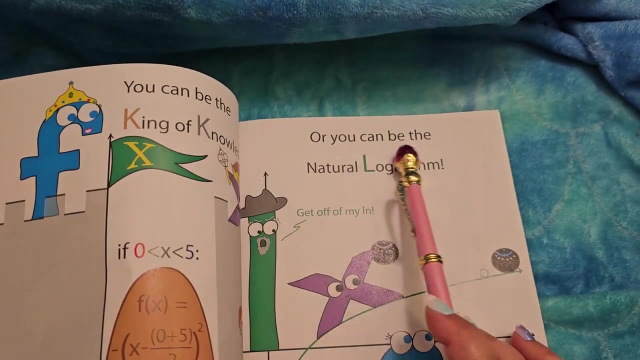 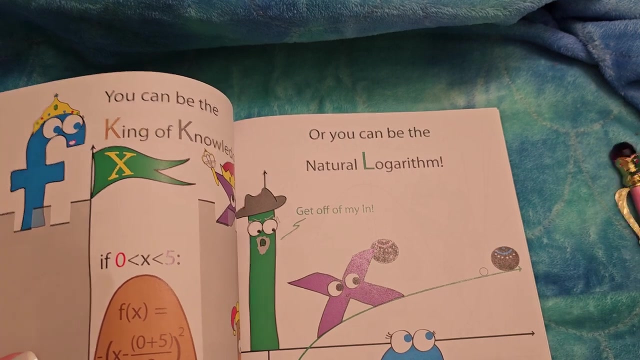 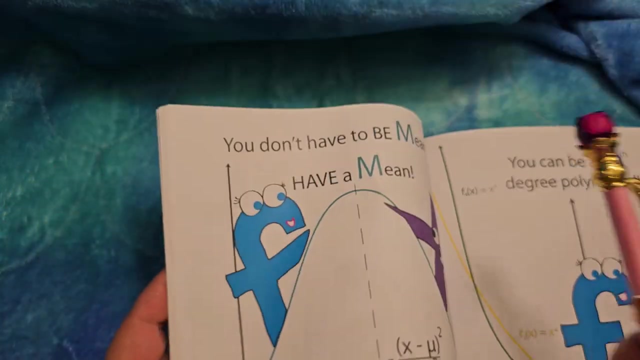 that's how that works. you can be the king of knowledge- oh, look at all of this math and look like the K is a jester- oh my goodness, poor jester. or you can be the natural logarithm. get off my land, Ellen. oh my goodness, so funny, you don't. 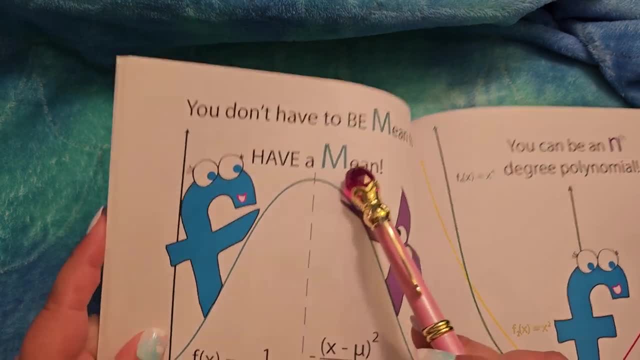 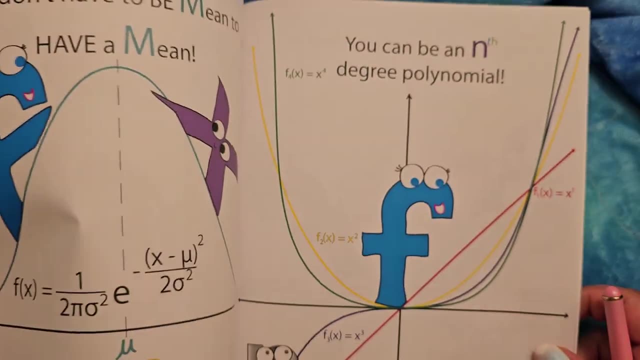 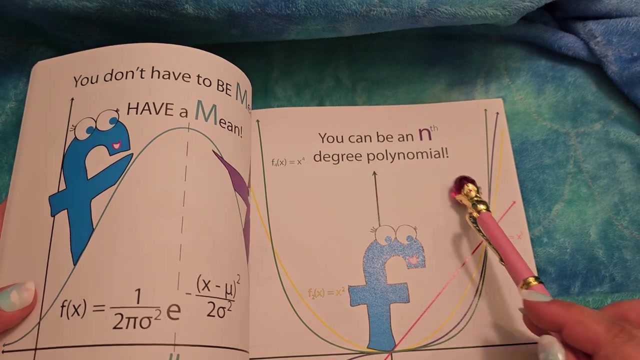 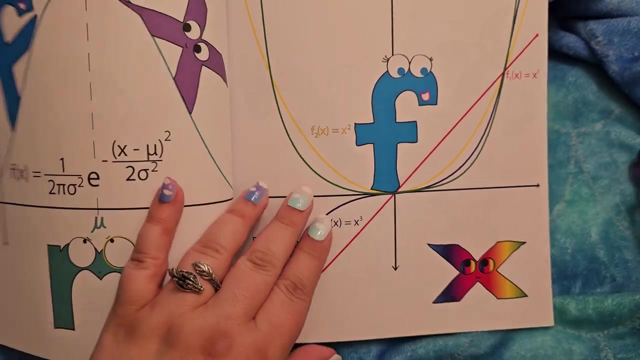 have to be mean to have a mean. oh, look at that grumpy M. yeah, mean is a kind of way of averaging something, not gonna really explain that. oh, you can be an nth degree polynomial. that is one way to get an n. so here's little n. he's like: look at all those colors. he's all rainbowy. how fun you can. 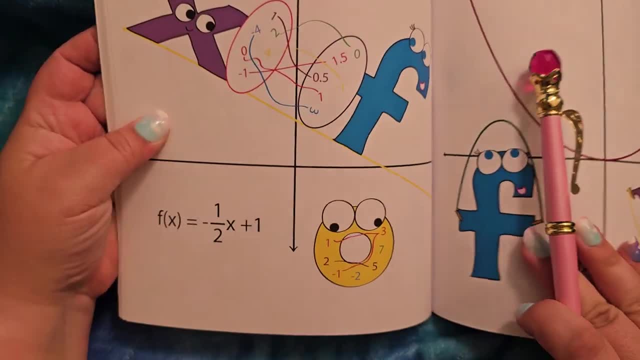 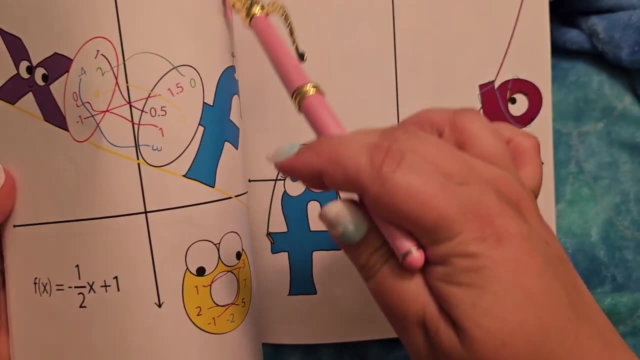 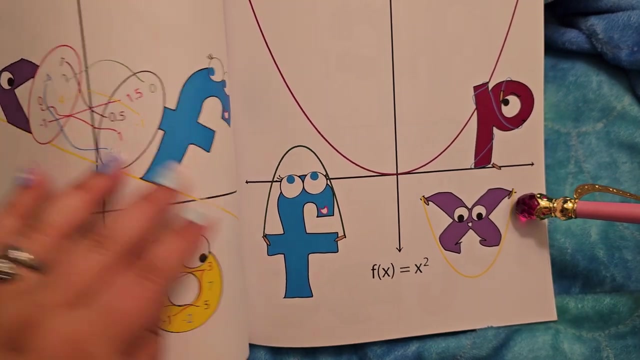 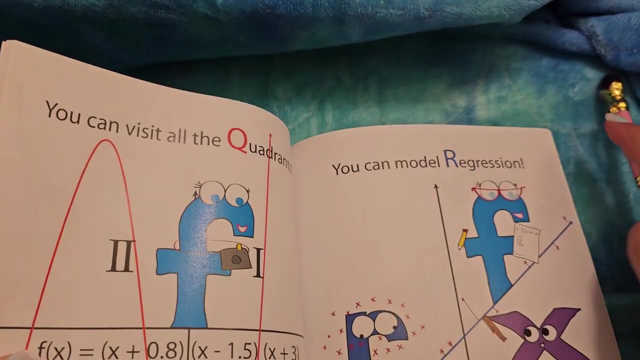 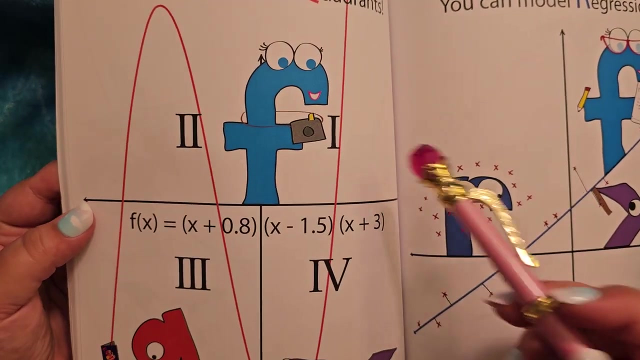 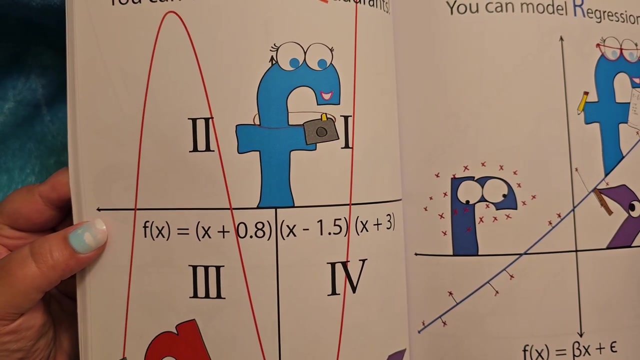 be one to one. look at that mm-hmm. or you can be a parabola that shapes called a parabola. oh, the P looks unhappy about this. this jump rope. here you can visit all the quadrants: the Q, one, two, three, four quadrants. oh no, it's an expired passport. 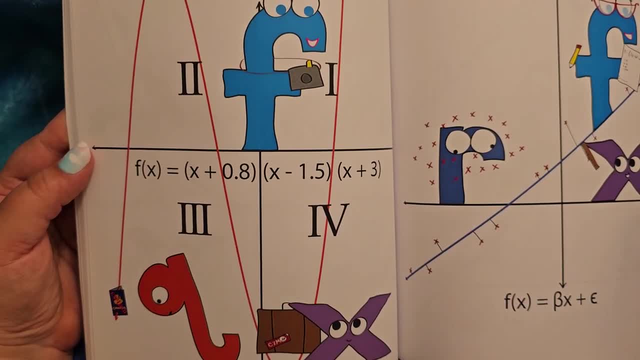 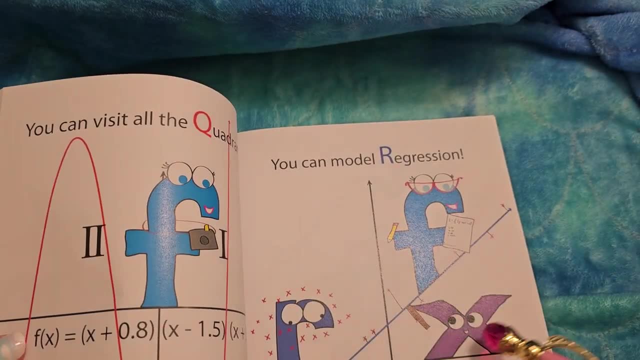 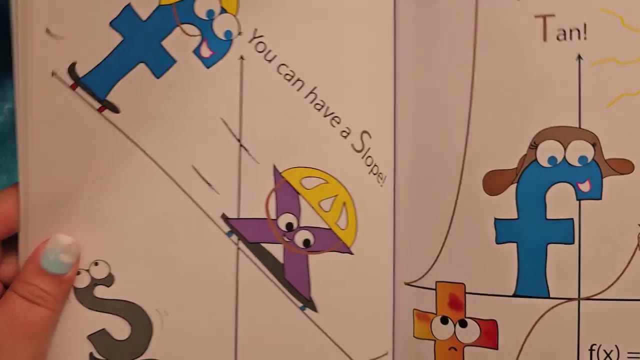 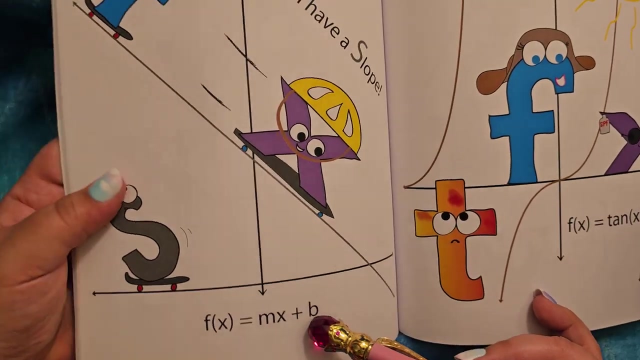 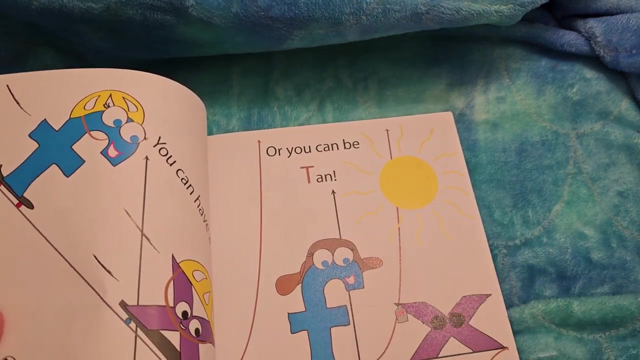 expired. four Q: look at little little down. you can model regression. so that's a nice little symbol down here. we're all the way to s. you can have a slope or you can be tan. oh, that's funny. a little joke with the Sun. tan has is a math term to not just how you get with the Sun. that looks like poor. 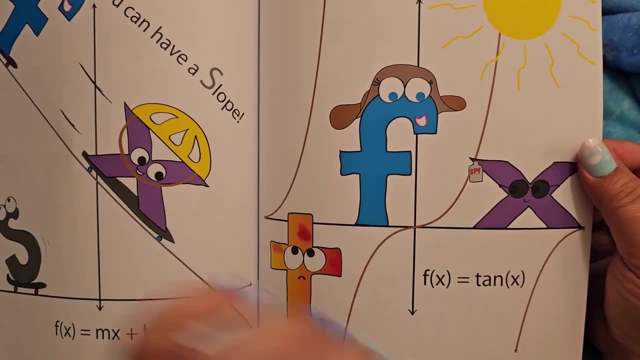 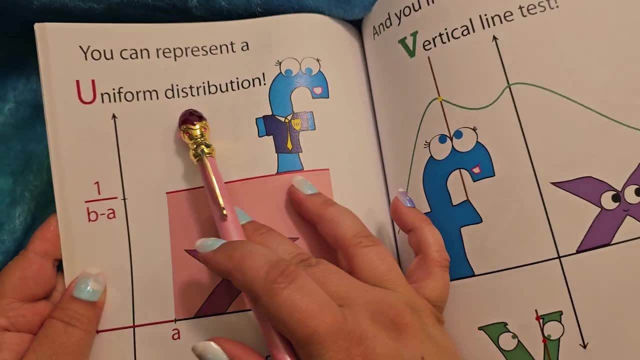 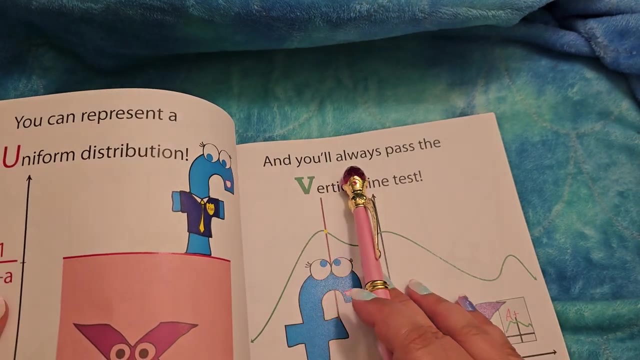 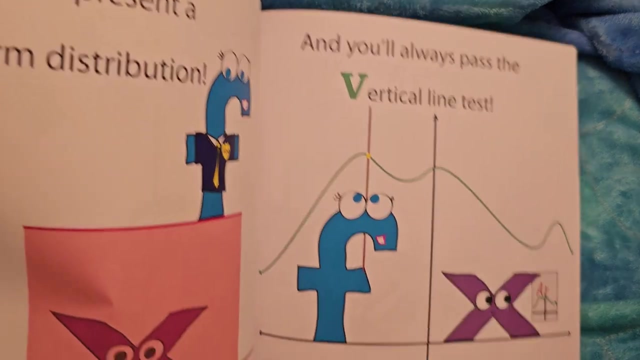 TV has a sunburn. you did to have some sunscreen. you can represent a uniform distribution. well, you looks a little unhappy down there and you'll always pass the vertical line test. I'm not sure exactly what that test is, but we'll see. here it is. we've got an eight plus. oh no, the. 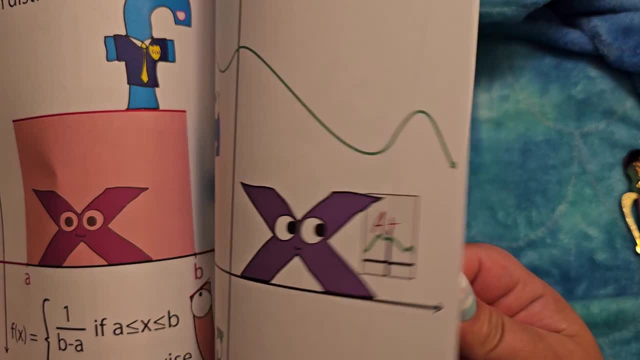 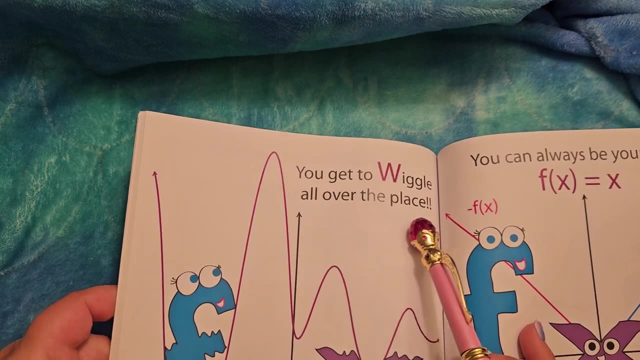 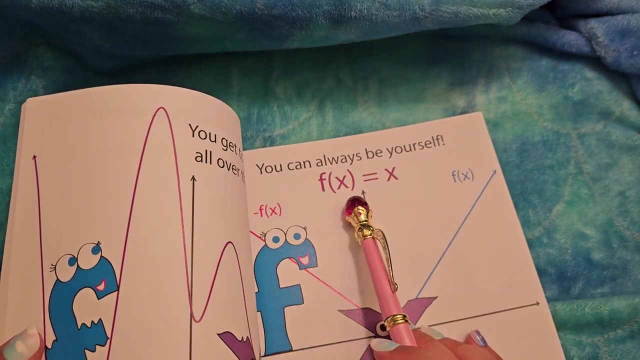 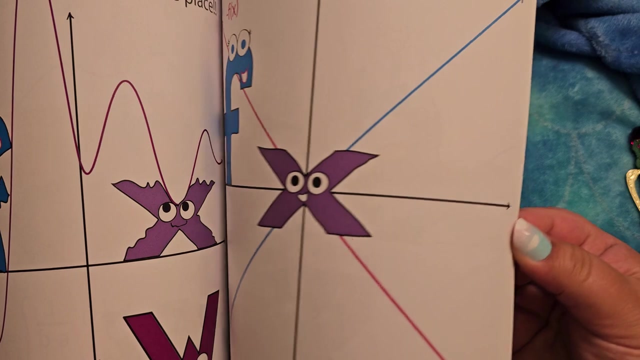 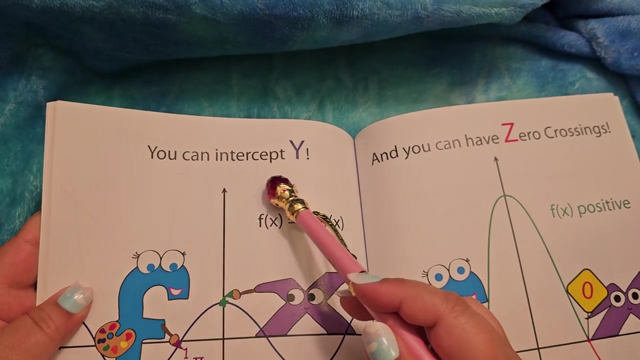 V has an F. he did not do well on that test. you get to wiggle all over the place. look at it, we don't. equally, you can always be yourself. so the function of X to X soup. all right, we're almost to the end of the alphabet. you can intercept why. oh no, they got paint on why. 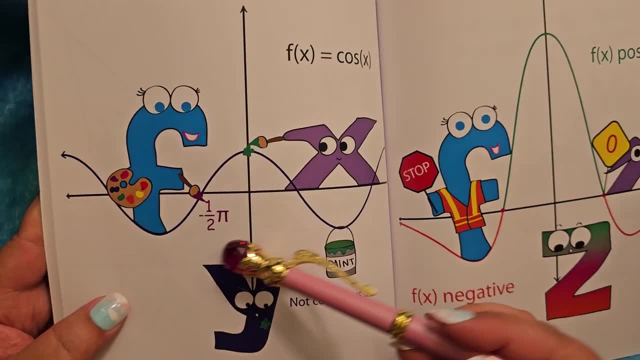 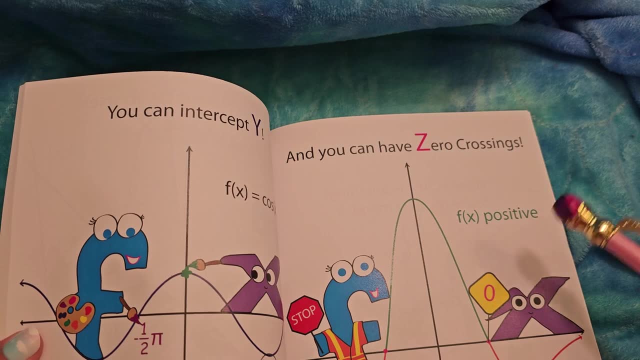 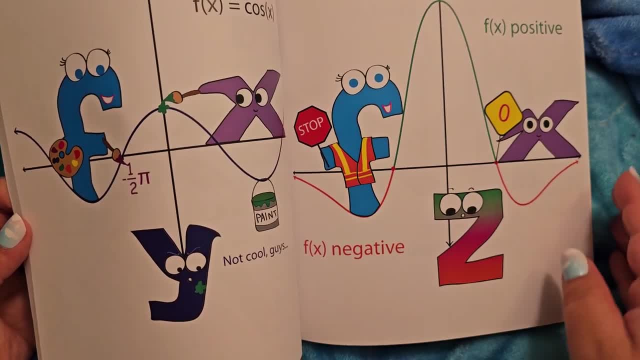 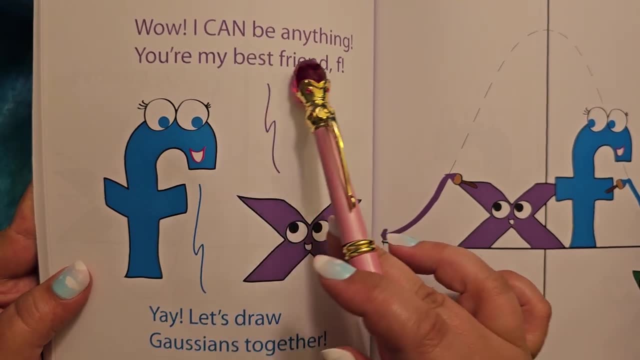 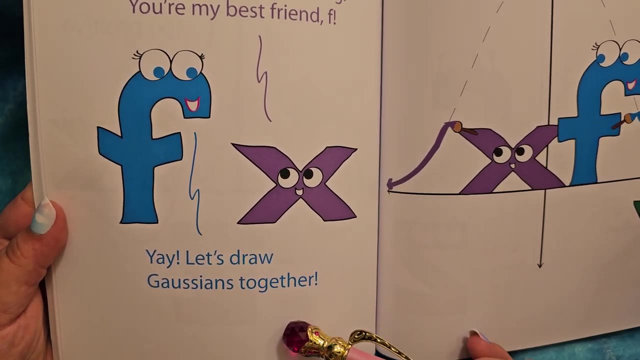 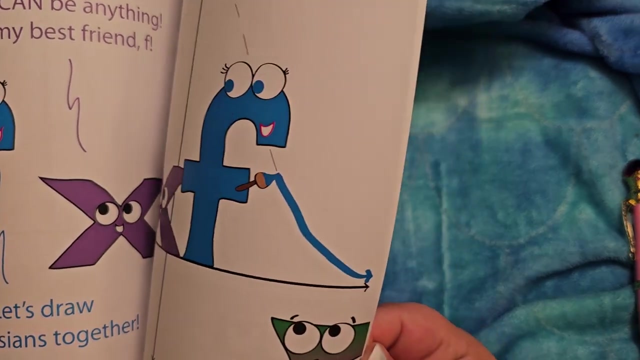